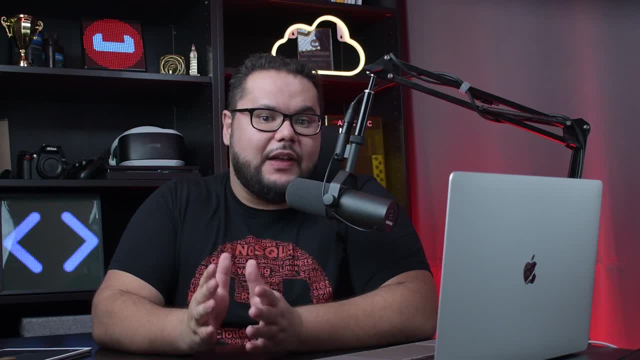 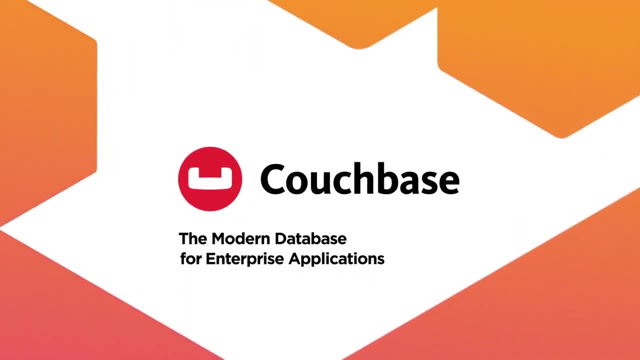 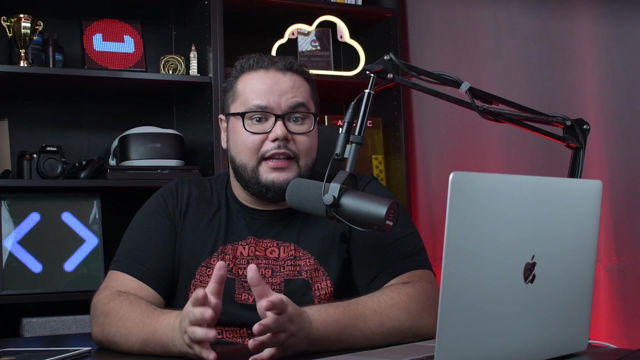 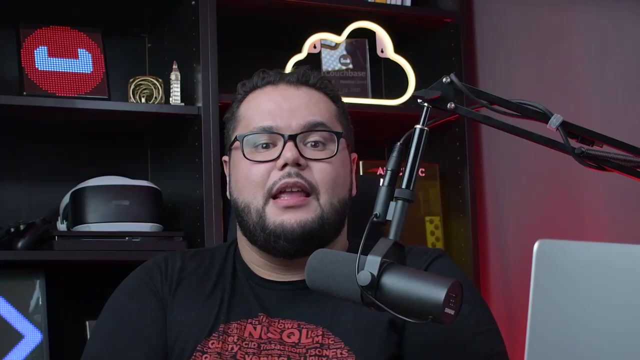 about how Couchbase did it and how it plays a significant role in performance. Let's get started. The first challenge while building a distributed database is to decide how to distribute the data between nodes right. Those subdivisions or subsets of data are called shards In many distributed 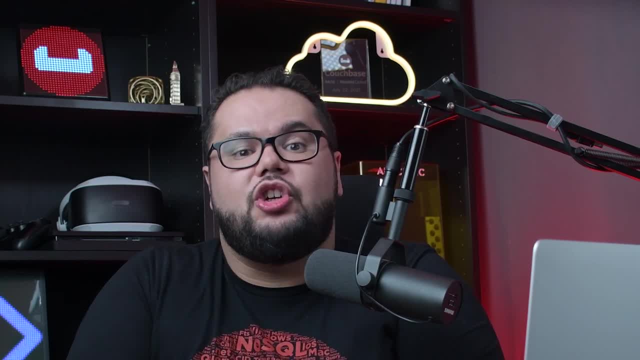 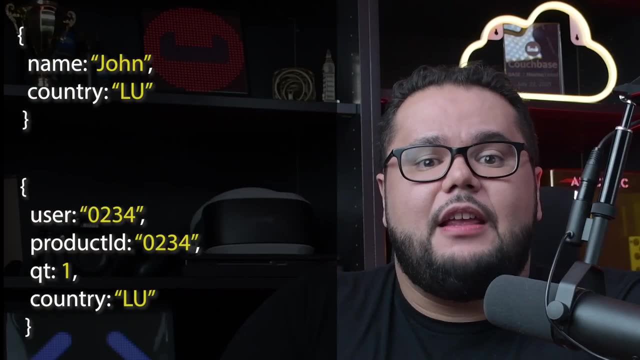 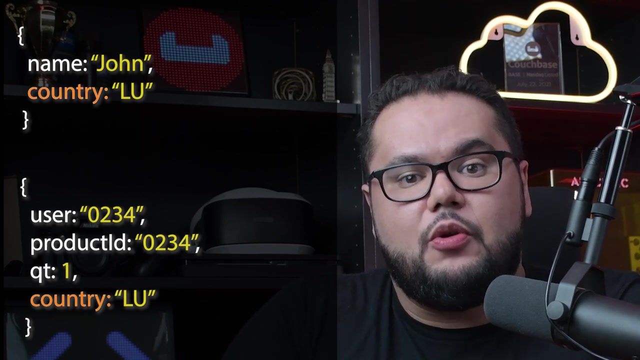 databases you have to specify a sharding key, which is usually one of the attributes of your document. But here is where it becomes a little bit tricky. Say, you need to store users and orders and you pick countries As the sharding key. over time there's a good chance that the China and the India shards will. 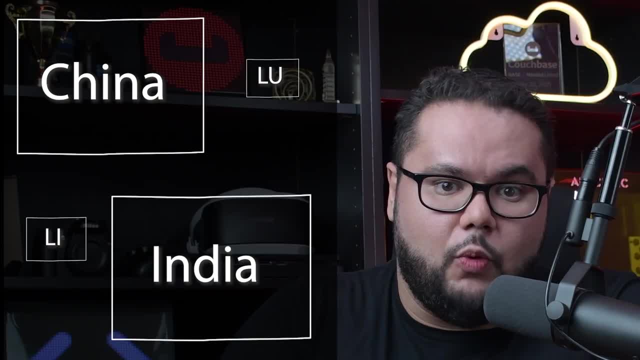 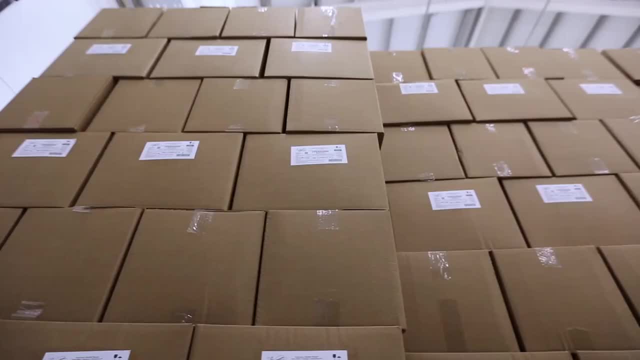 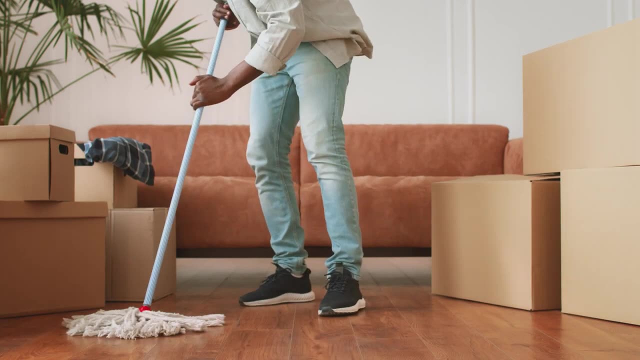 be much larger than the Luxembourg and Liechtenstein ones. As a shard cannot be subdivided, the server holding the China and the India shards will be overloaded, while the one holding Luxembourg and Liechtenstein will most likely be sitting there doing nothing. 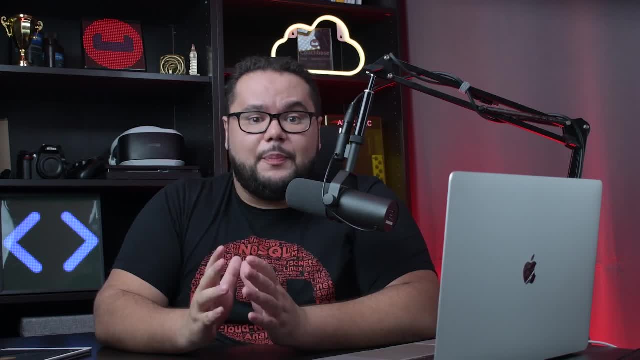 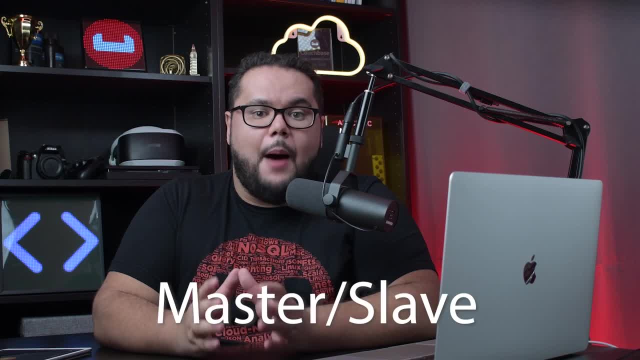 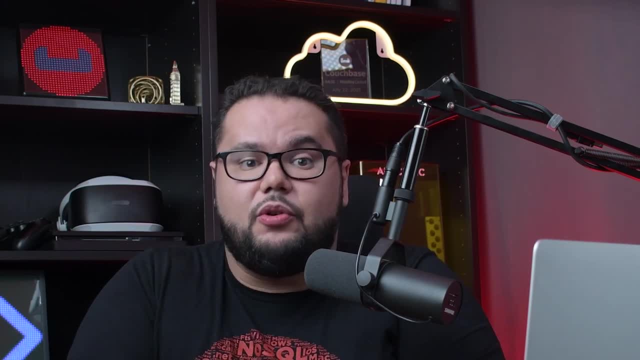 maintaining the map of shards. This is what we call a master-slave architecture. This approach makes the database implementation a lot easier, but introduce a few other methods. For example, requests have to go to the master and then to the slave, which will impact your 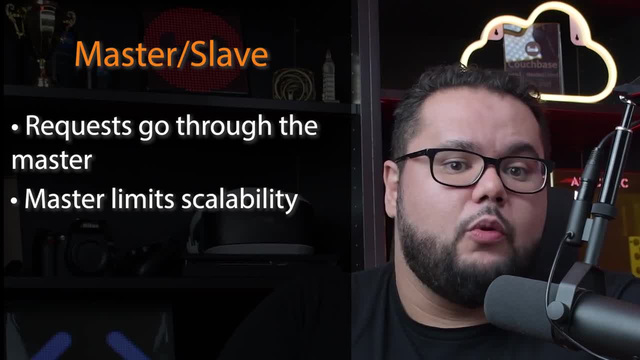 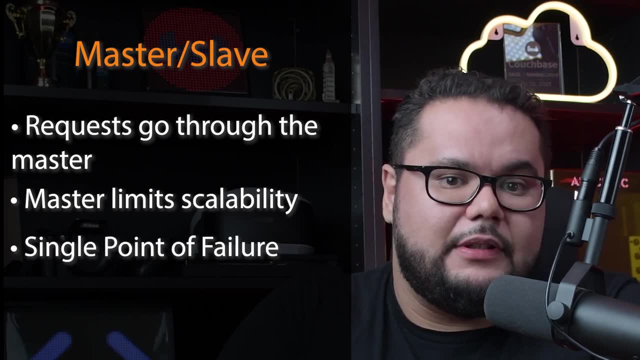 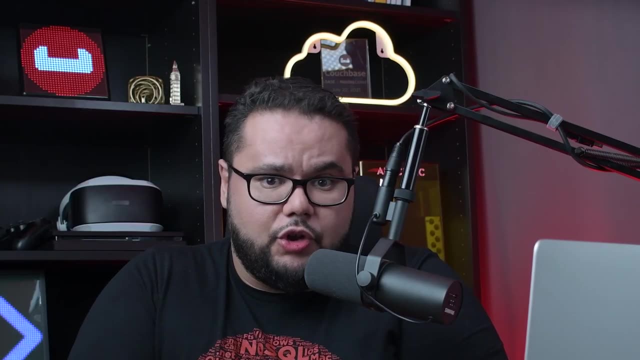 query performance negatively, The master node will naturally become the bottleneck and also limits the scalability of your cluster. When the master goes down, the database becomes unavailable until a slave gets promoted to master. Now let's talk about Couchbase's approach, which is significantly different. First, Couchbase has a fixed number of shards: 1,024,. which in theory limits the maximum number of nodes that a single cluster could have to 1,024.. But in practice it's hard to see one single database with more than 100 nodes in it. This default number of shards also prevents them from growing larger than what a single node could. 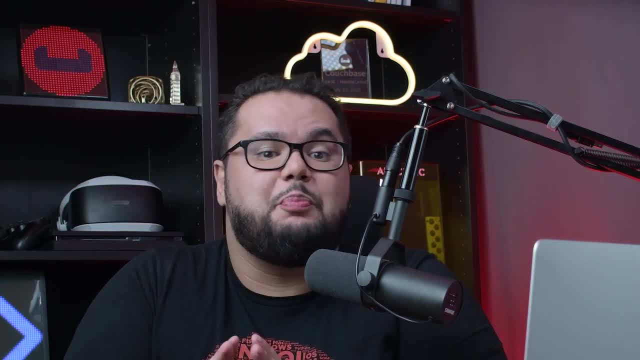 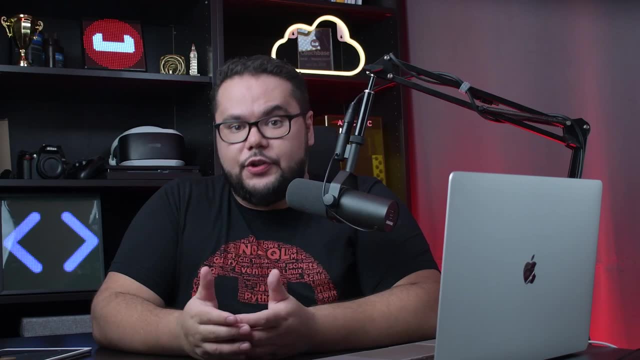 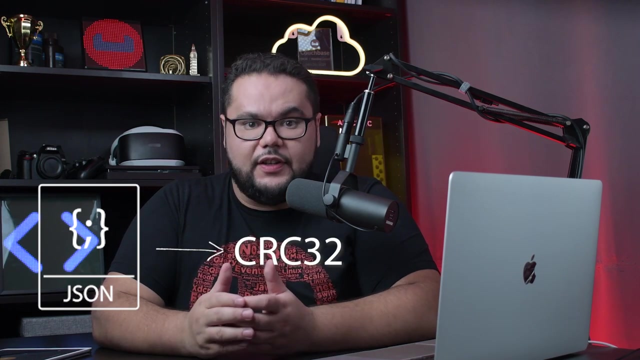 handle. Worth highlighting that these shards are transparent for developers. From their point of view, they see just one big database. Here comes one trick: Whenever a new document is added, Couchbase hashes the document key using an algorithm called CRC32.. According to the output,